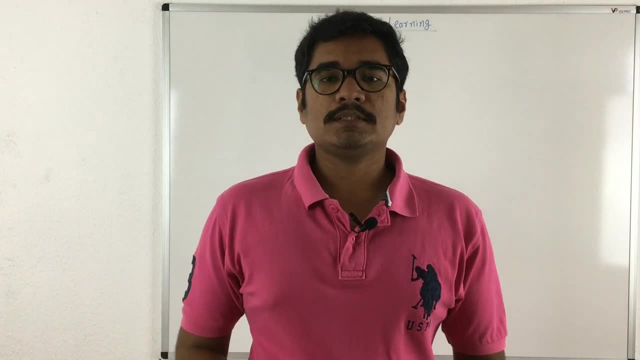 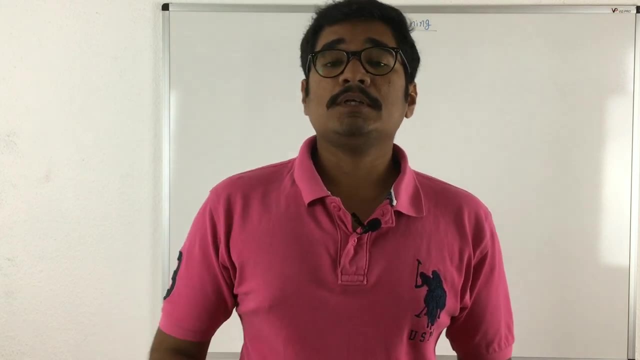 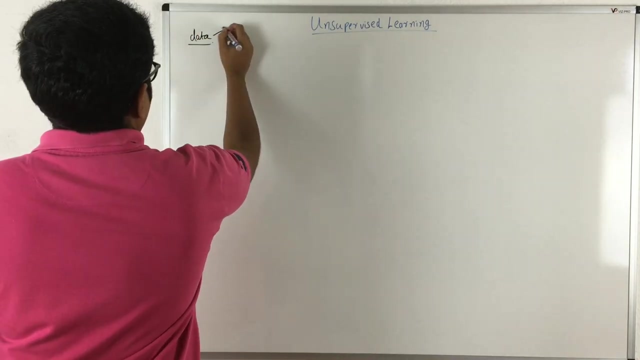 algorithms we learned in that. So in all this we had the data as in labeled format, and so the discovery process, that is, the information discovery process, was in a supervised manner. So here also we start with basic as the data. So data in its original format has two forms: 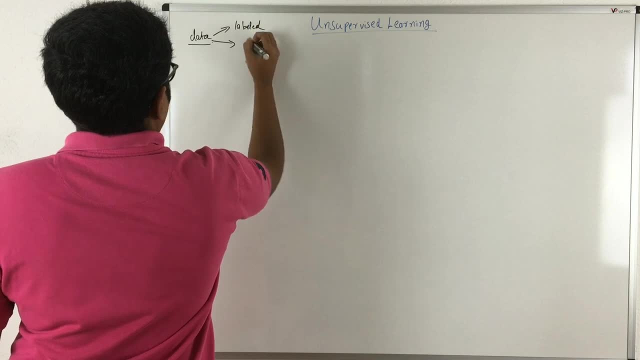 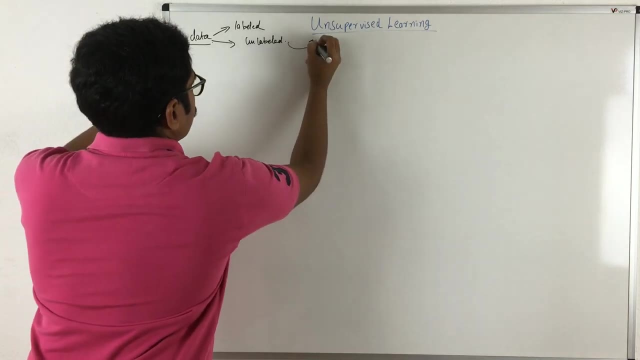 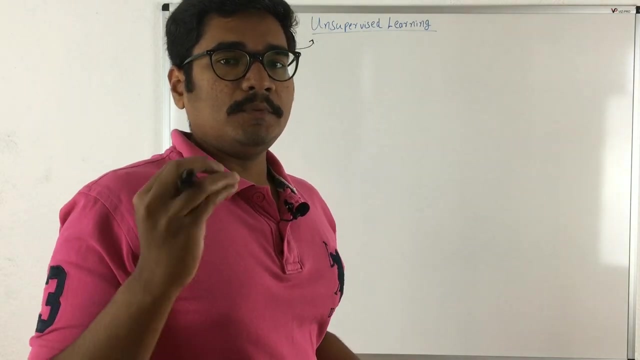 that is, first is labeled and second one is unlabeled. Okay, so unlabeled data we mainly use in supervised learning means, although we have data in both format- labeled as well as unlabeled- but in supervised learning we mainly use the unlabeled data. So what you have, 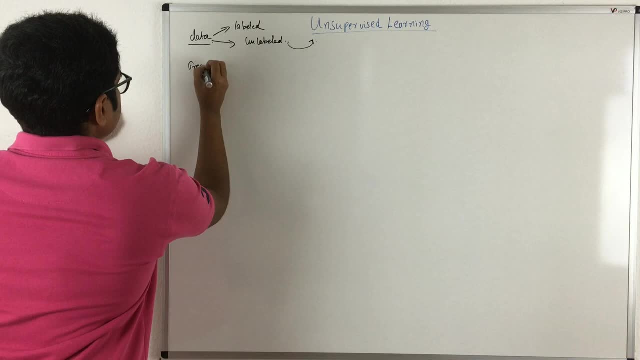 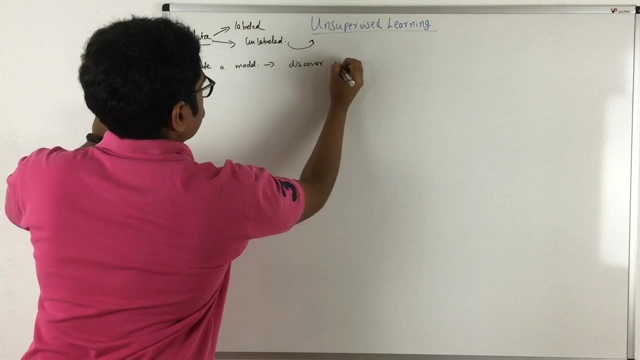 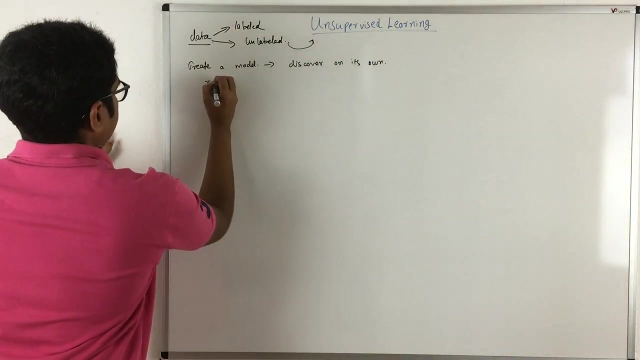 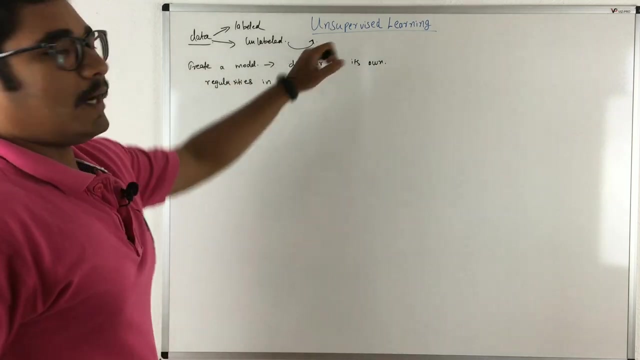 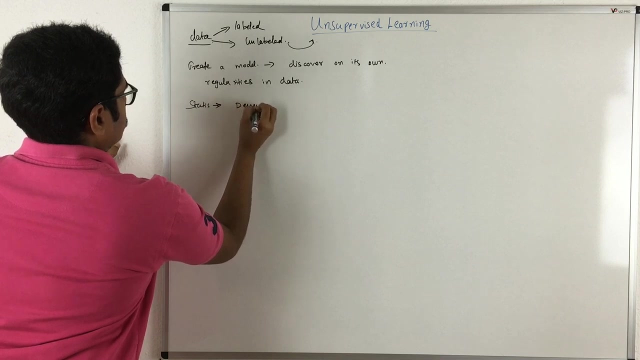 is we create a model and allows us to discover on its own, that is, for new patterns or new features. So it basically finds the regularities which is present in data, Now unsupervised learning. in statistics It's called as density estimation, So basically where you have dense points. 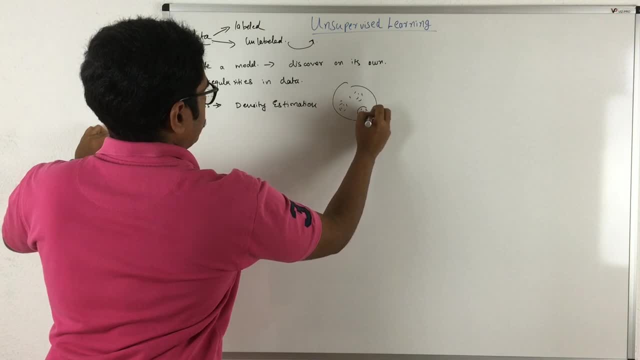 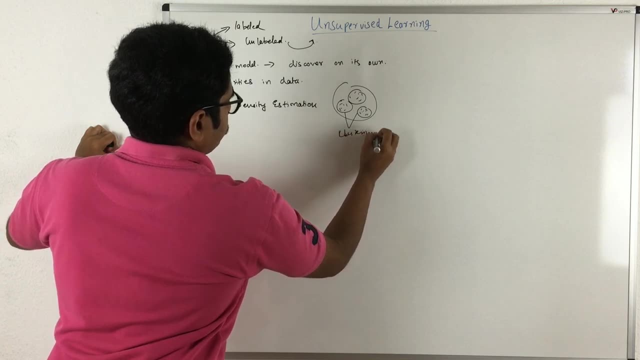 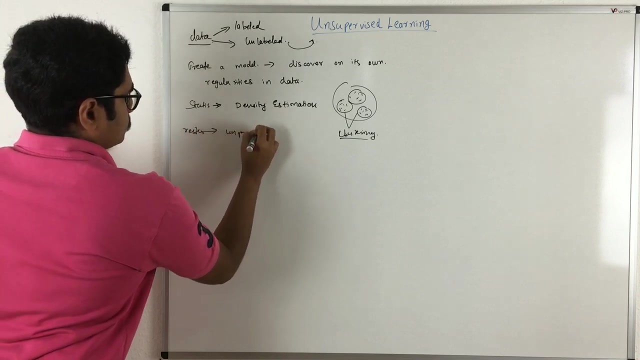 and you try to estimate the regularities in that particular pattern. So this is basically an application called as clustering, And so the results you get from this are basically unpredictable. Whereas in supervised learning what you had is you had accurate results. So here in unsupervised learning, you get very less predictable results. means 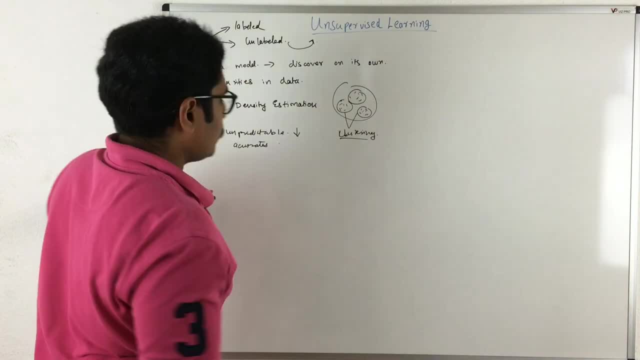 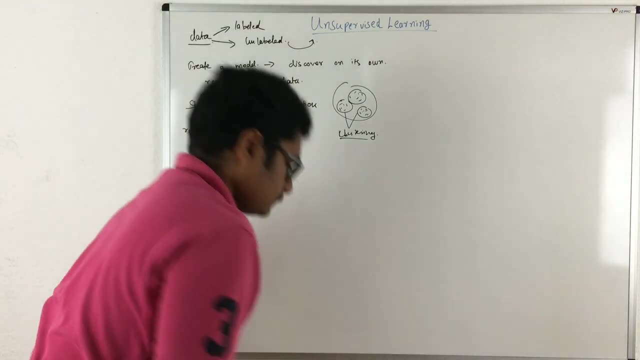 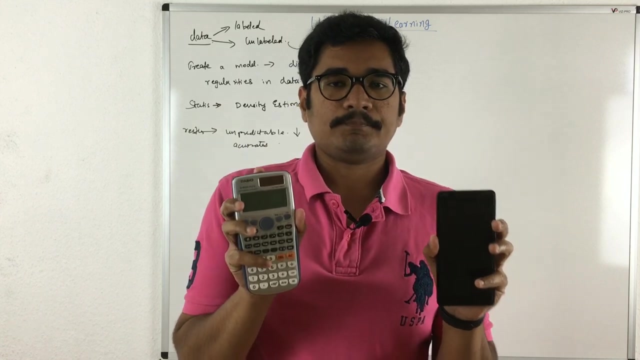 either you will get the result as correct or it will go for a toss. So any of that case is possible here. Now to understand this, Let us take an example of say: these are two electronic devices- Now this is a smartphone and this is a calculator. Now, if I give to a person or say, for a 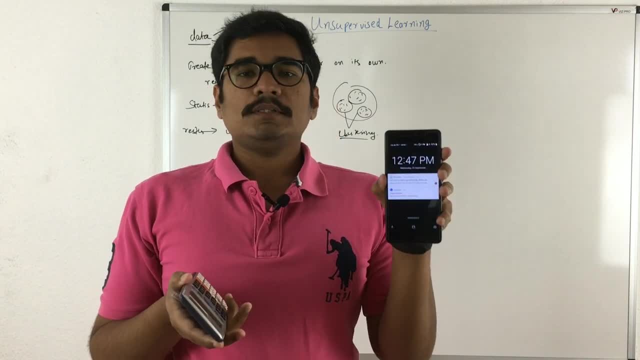 child if I have given this phone. Now, if I give to a person or say for a child, if I have given this phone, So they know that this is a phone And they will know that this is a phone, But he or she 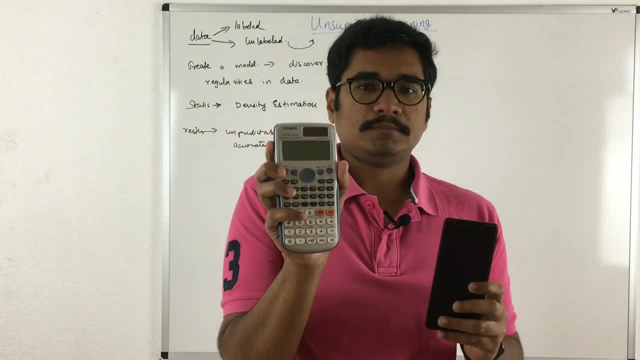 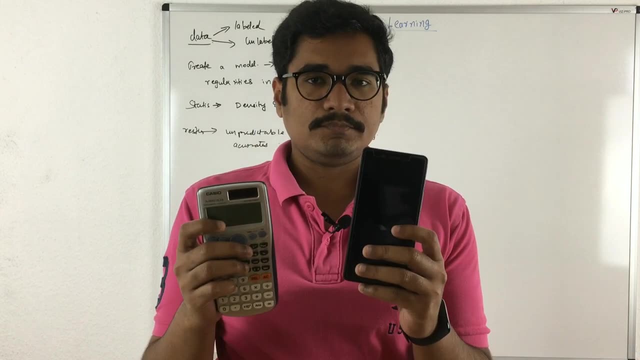 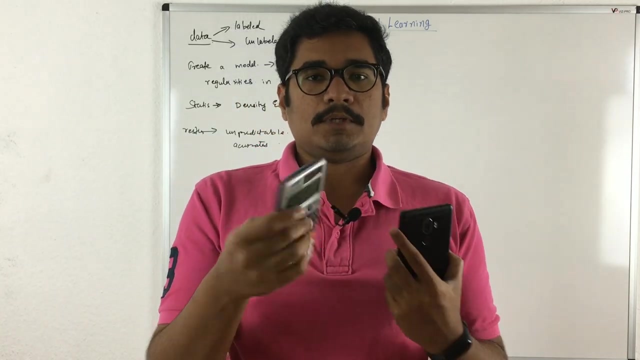 may play with it daily. Now, if I give this, that is calculator, but they'll find like it's of the same size but it doesn't look similar as of this. Now, this is what you can see as a single glass piece. Then there is a front camera, then you have a back camera, So they will try to. 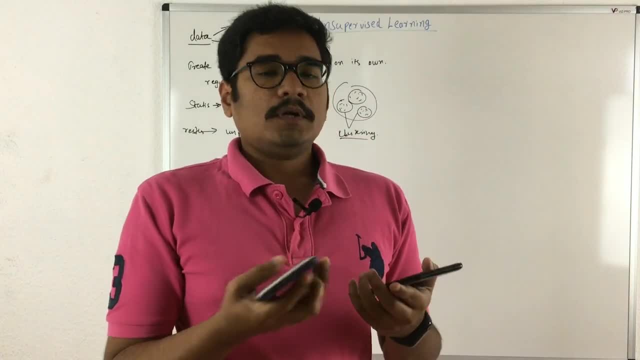 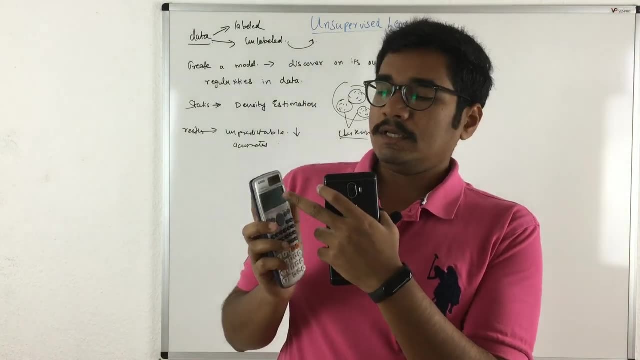 see at the back side, but it looks different. Now, what makes it different is that you have a small, smaller screen. first, will identify that it has two screens, that is, this one and this one. then there is no camera here, or they will try to make the analogy that this will be. 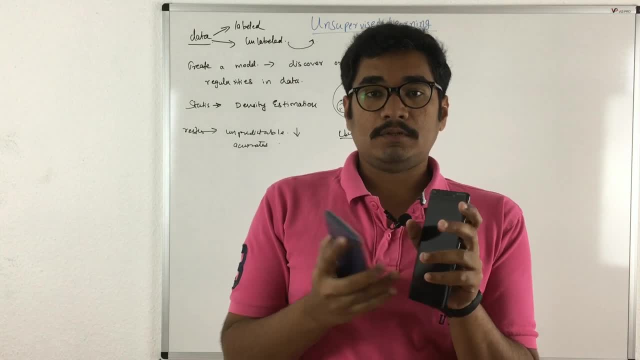 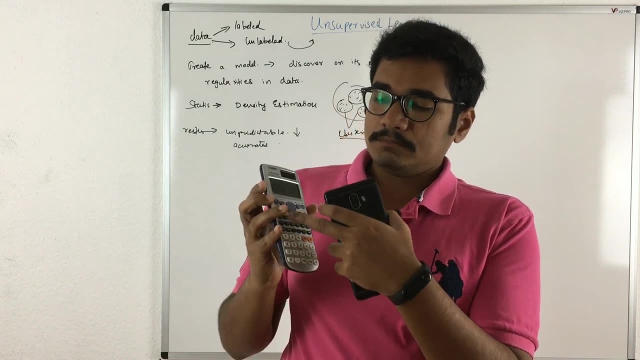 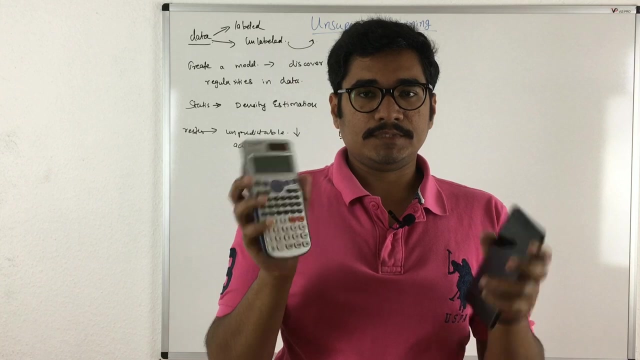 the camera, something like that. then it has more buttons as compared to this. they have more colorful buttons. then the color or the texture is different. then you have different small buttons of different format, so something like that. so what you do is you try to identify the patterns which are present in both of these items and then you finally categorize. 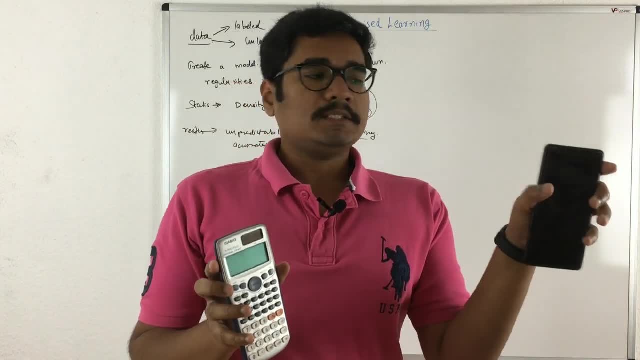 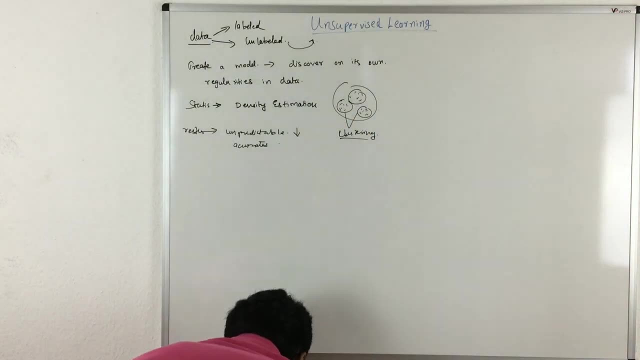 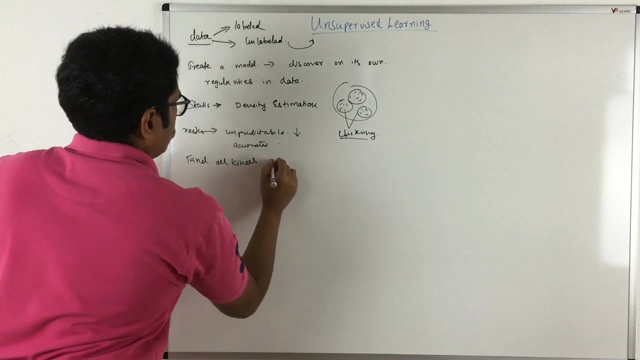 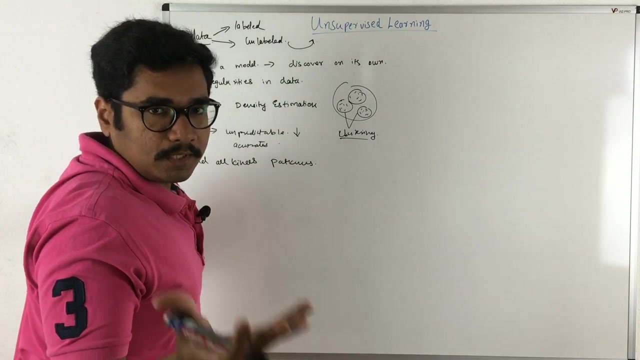 or you put into different, separate instances, like this is a smartphone or this is calculator. so something like this happens over here. So it tries to find all kinds of patterns. So if you have not told them like it has different kinds of buttons Or something like that, but they'll try to identify different kinds of features means 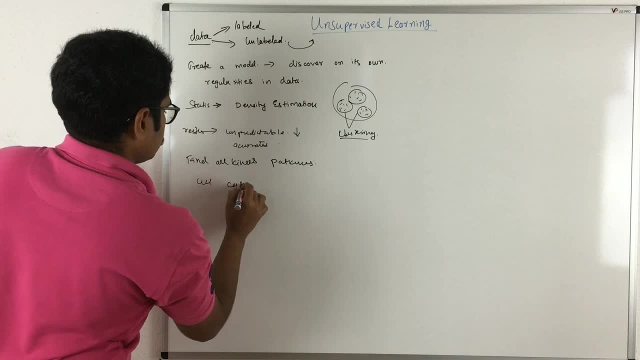 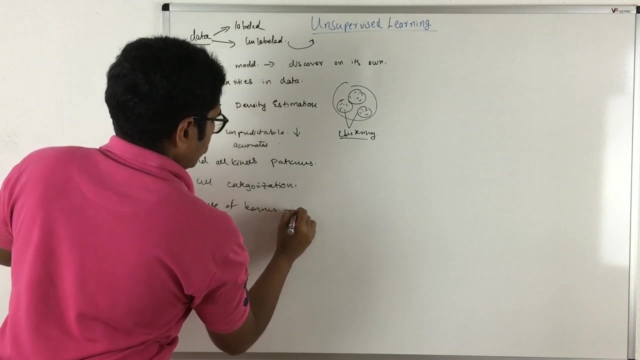 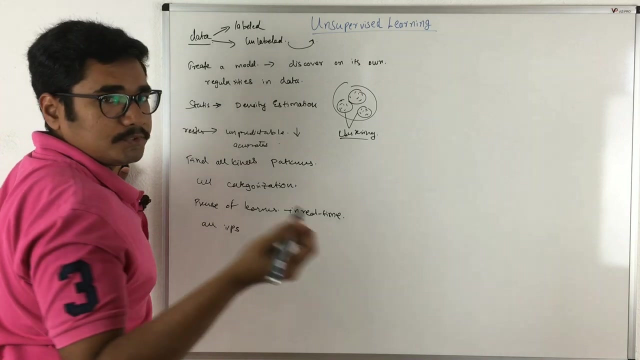 all types of different features and it will be all used for categorization. Now, this type of clustering is mainly done in the presence of learners. That is in real time. So all the inputs which are there or which you get. So all the inputs which are there or which you get. 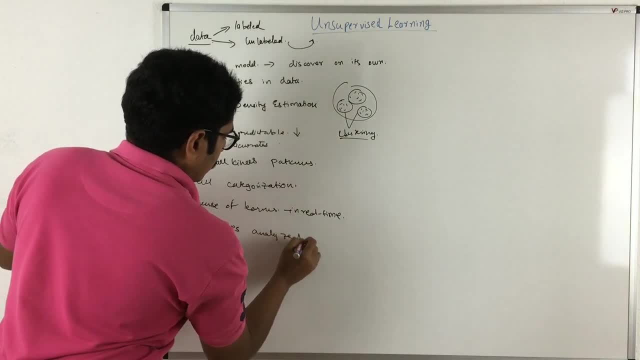 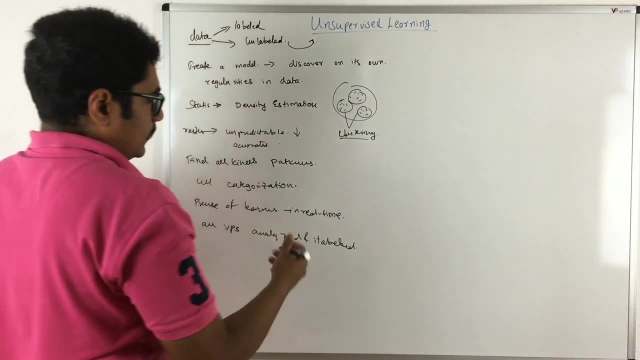 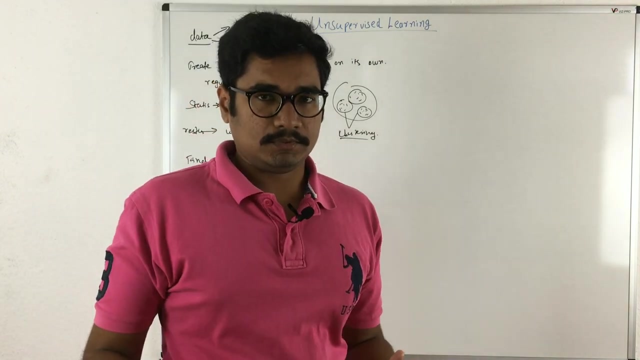 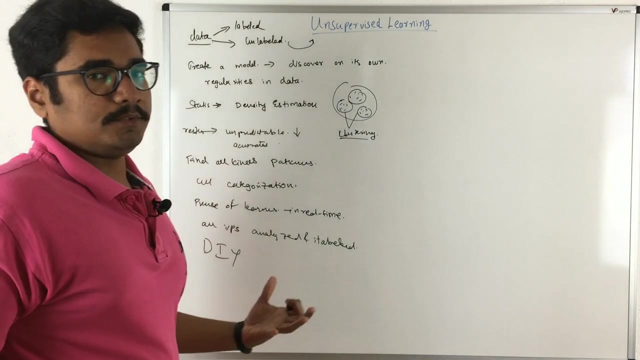 Is analyzed and it is labeled in the presence of users or learners. So essentially this: there is no particular external factor or external supervisor in order to guide your process. So what it is, you try to learn from your own, So it's kind of a do it yourself activity. 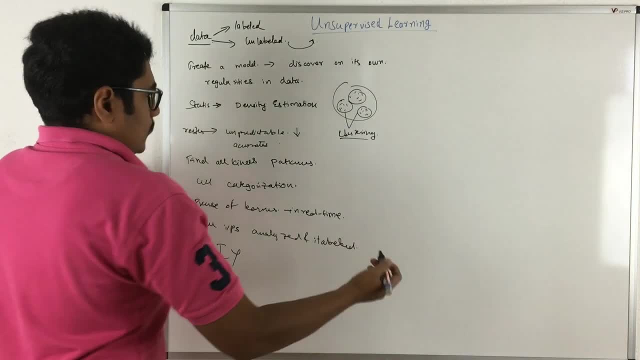 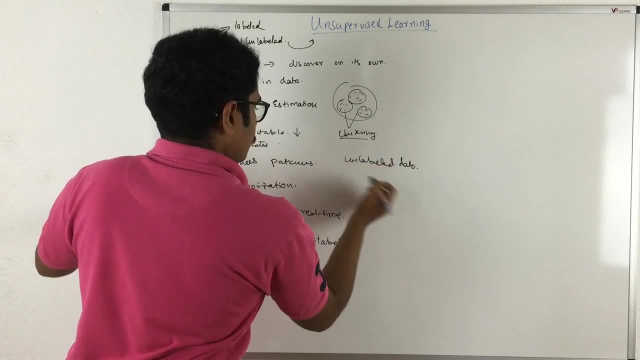 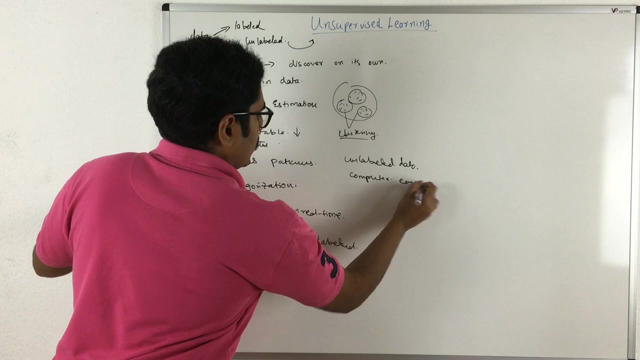 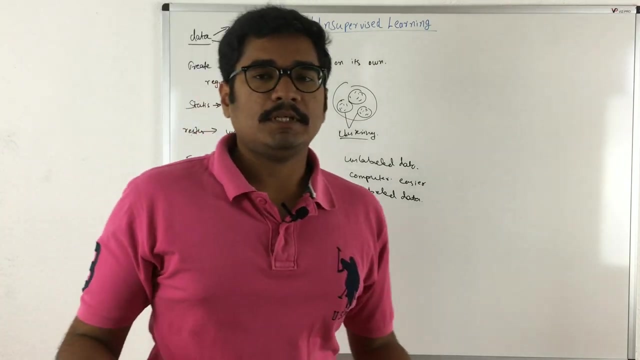 You can just understand something like this. So and one more thing is To get unlabeled data From a computer, So you get mainly data from computer is far easier as compared to label data. Now say, for example, some person is there and he is hungry and he says like, get me anything. 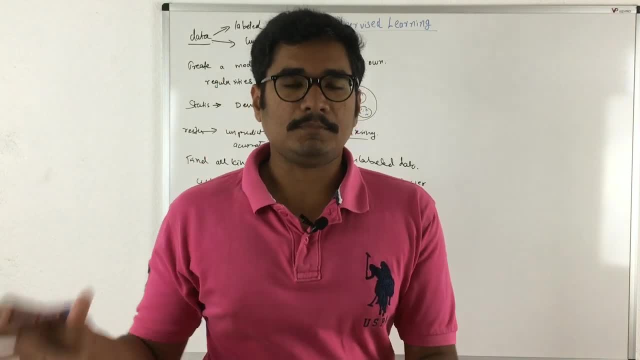 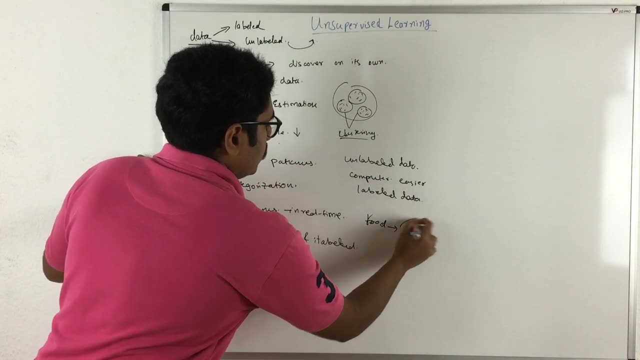 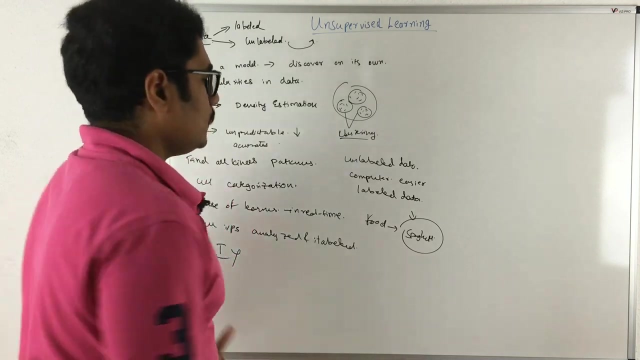 to eat. There is no particular thing he mentions. But if he mentions like: I want spaghetti, So food is one particular kind of data. So you label it as spaghetti. So that becomes labeled, So label becomes difficult to get in case of unlabeled data. 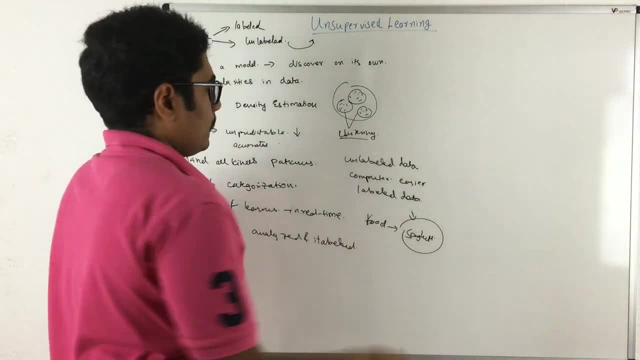 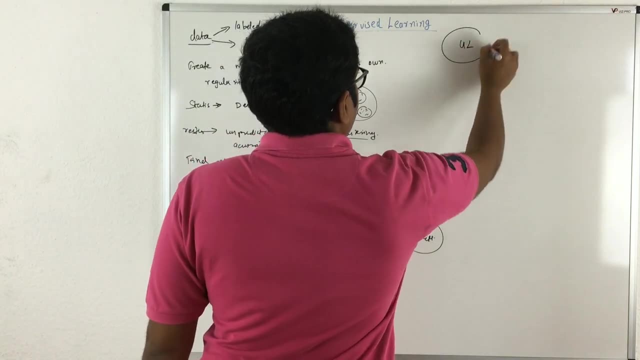 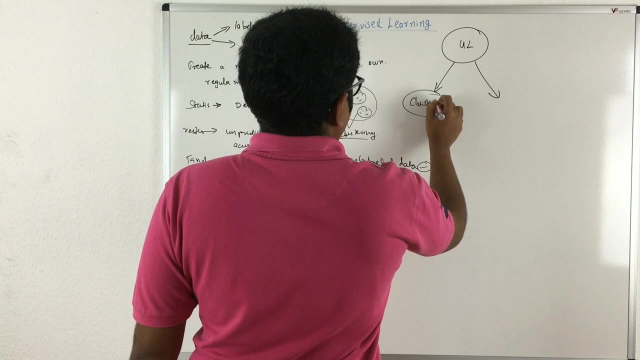 So that's in vast number, So you can get it at any time. So that is the main thing here, So you can get unlabeled data easily Now. secondly, you have unlabeled data divided into two categories. First, you have some clustering based applications and here you have associations. 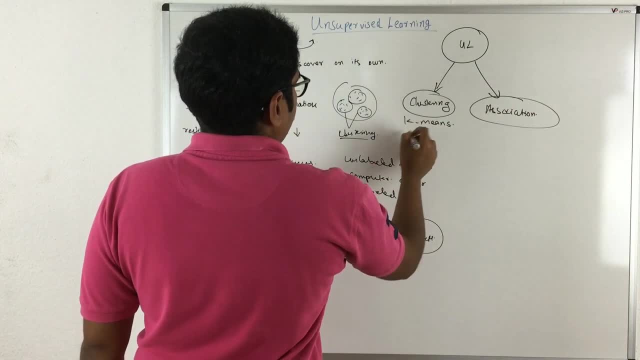 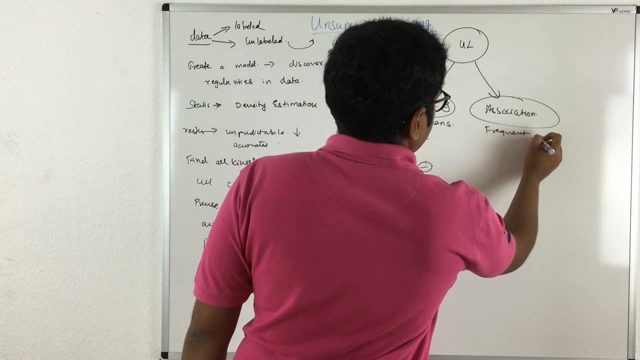 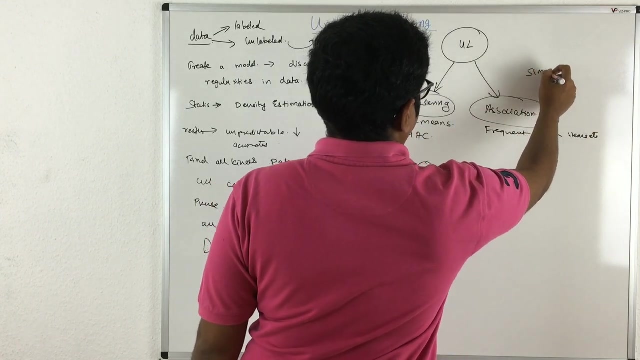 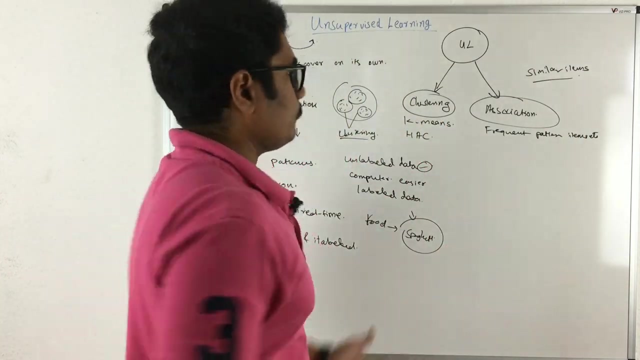 So in clustering you have some k-means algorithm, you have hierarchical clustering algorithm, something like this, and here you have frequent pattern item sets where you club similar items together. Similar items are clubbed together So that it's frequency is counted in that particular data set. 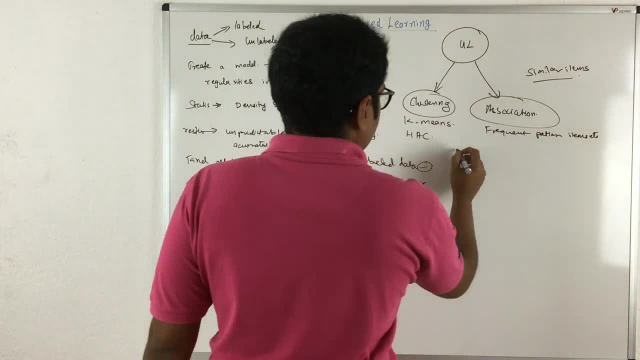 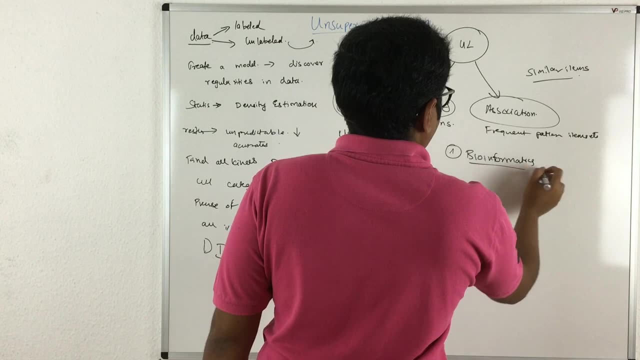 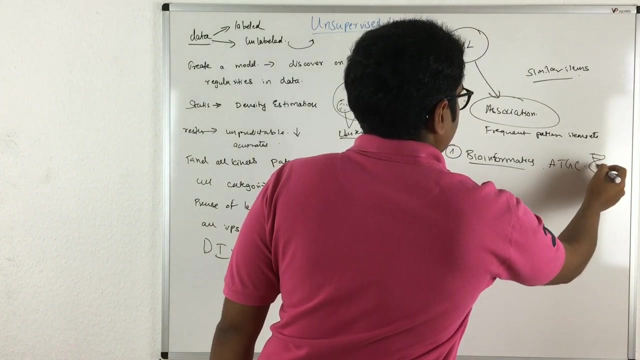 Now, unsupervised learning has got certain applications. So very first and foremost is in bioinformatics, where you have this genes present in ATGC format, that is, in DNA structure. So here you basically used for categorization, So it's used in genetic clustering. 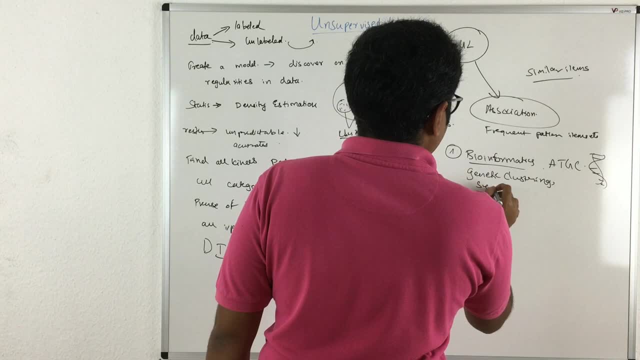 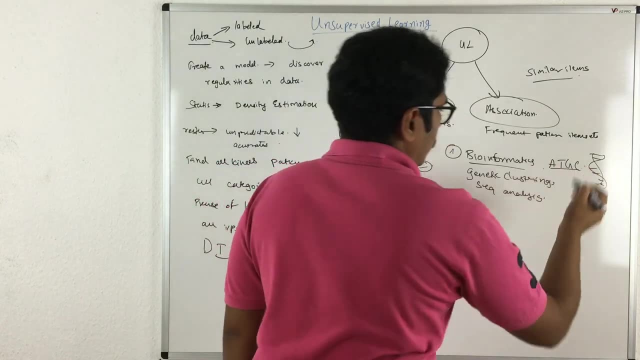 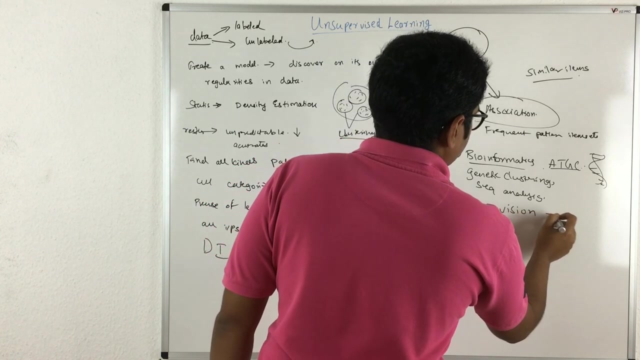 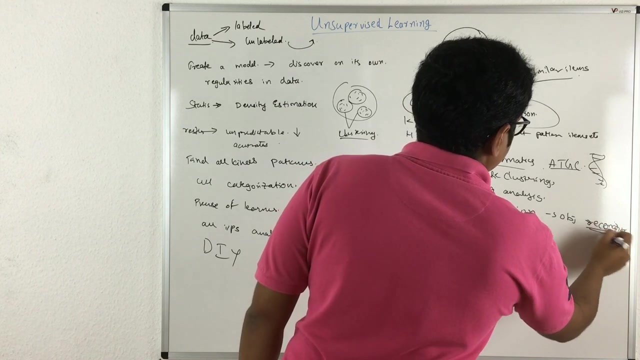 Also it is Okay in sequence analysis how the sequence appears, or after which character or which protein strand it basically happens. second is in computer vision you mainly used for object recognition. So in robotics mainly you have this application. third, you have in deep learning.